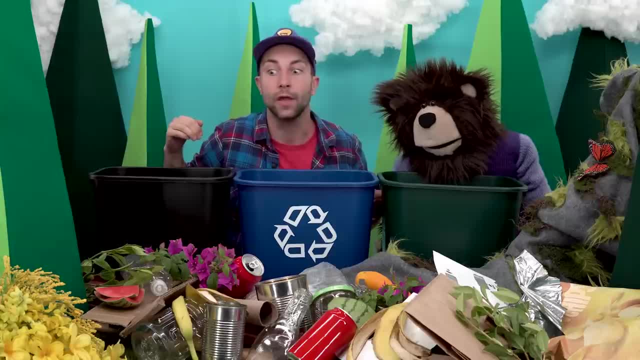 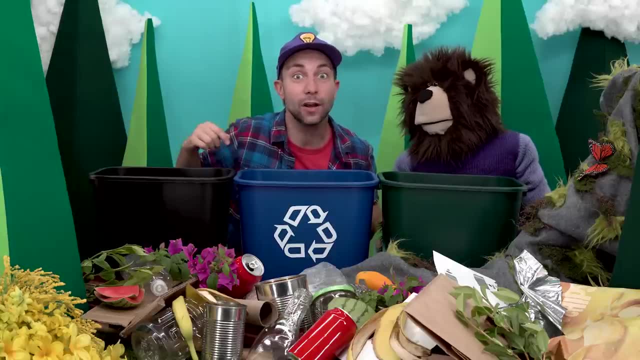 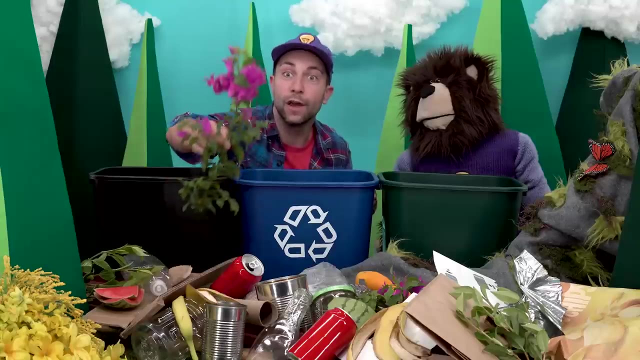 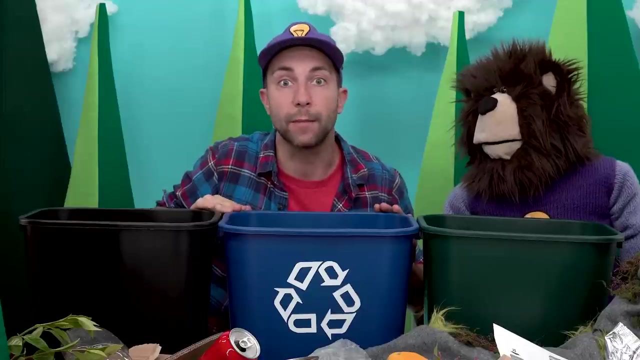 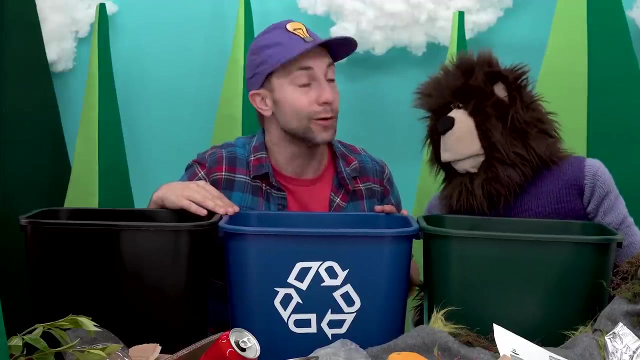 out here that can go in the green bin. you do so, do i? do you see anything that could go in there? that's right, these flowers can go in the green bin. okay, now let's talk about the blue bin. the blue bin is for recycling. isn't that neat? recycling is very important because we can reuse materials and make things. 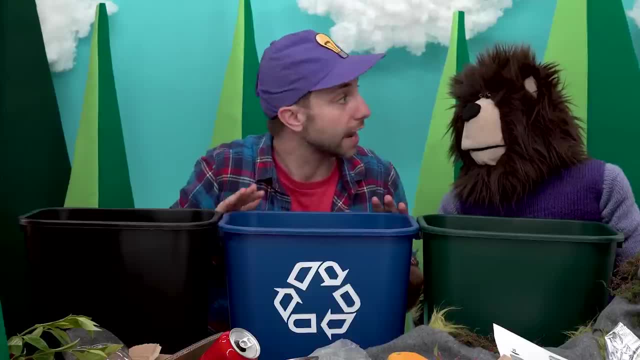 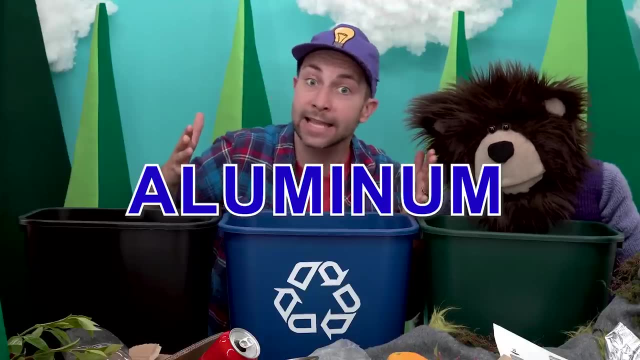 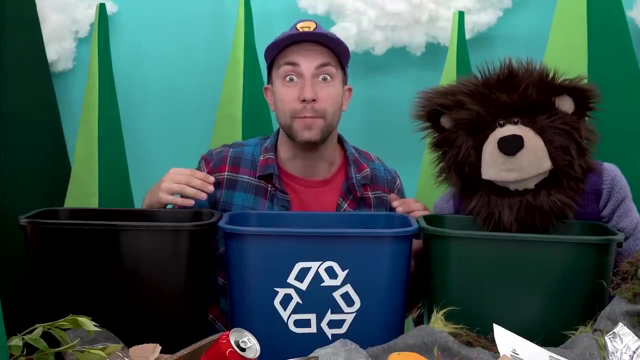 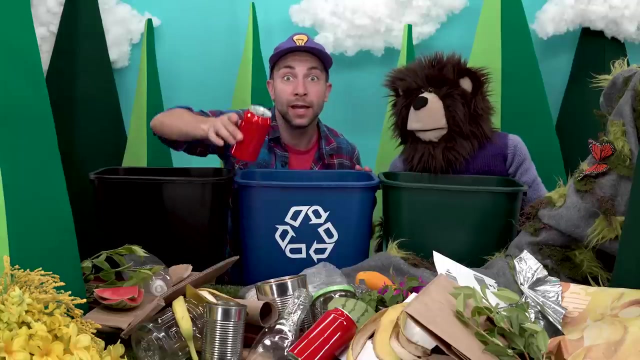 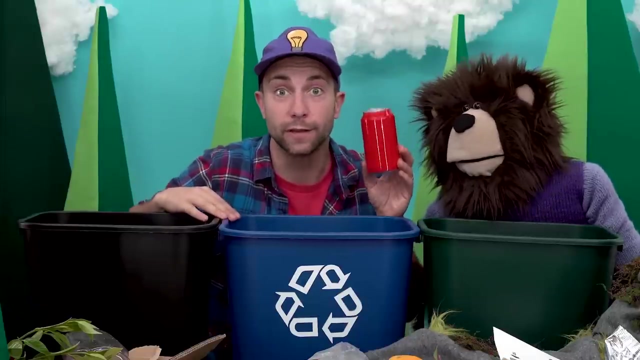 from them. so the things that can go in the recycling bin are paper, cardboard, plastic, glass, aluminum cans, tin cans. mayta, do you see anything out here that can go in the blue bin? what about this aluminum can? it's a pop can, or maybe you call it a soda can. this can be recycled, so let's put. 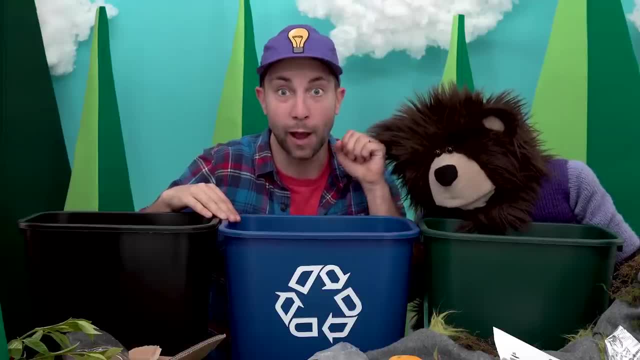 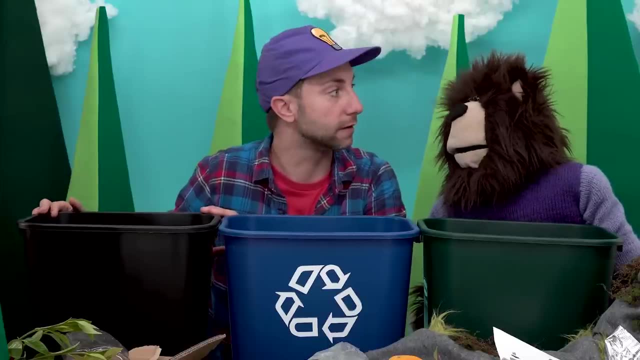 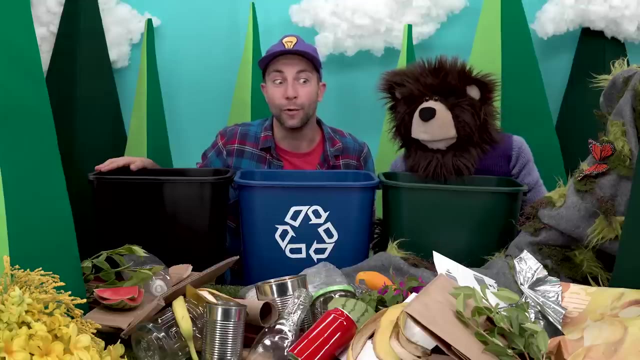 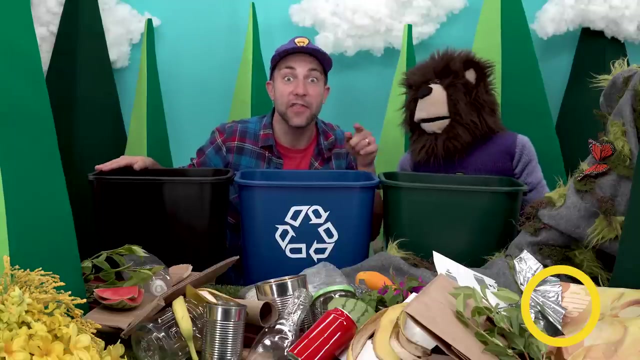 it in the blue recycling bin. all right, moving on to the black bin, this black bin holds everything else. it's all your trash. do you see anything out here that can go in this black bin? oh, do you see a chip bag way over there, mayta? do you see it? yes, that is a piece of trash, so let's grab it, all right. 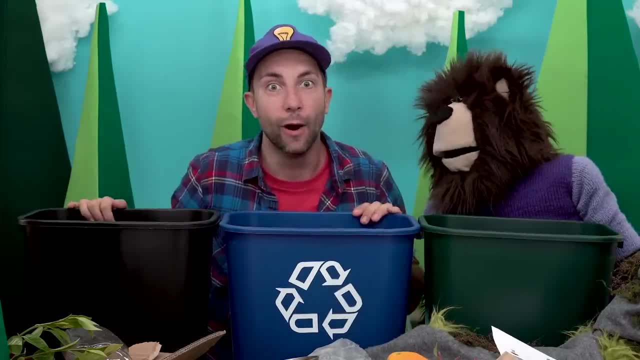 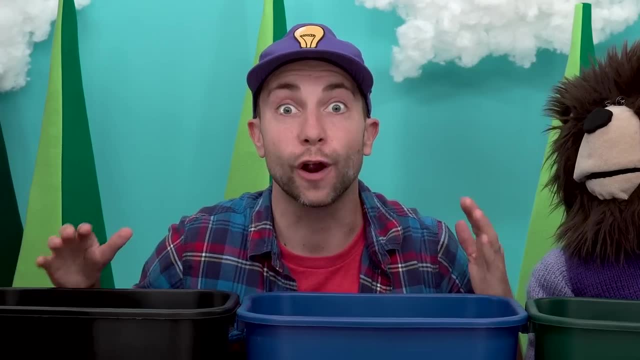 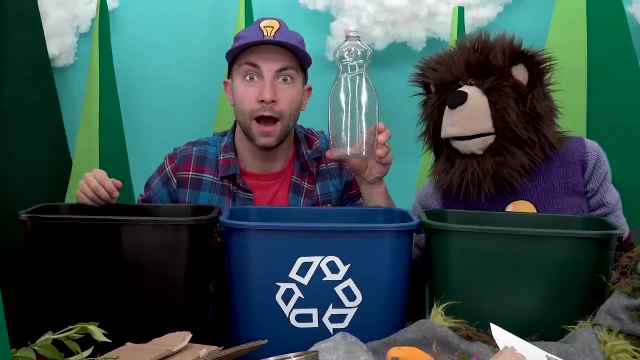 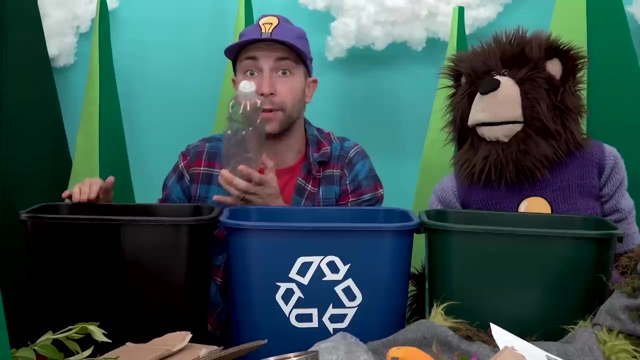 and we will put this chip bag in here. all right, so now you know what goes in each one of these containers. okay, so let's start cleaning up. oh, what is this? that's right, it's a plastic bottle. and does this plastic bottle go in the green bin, the blue bin or the black bin? 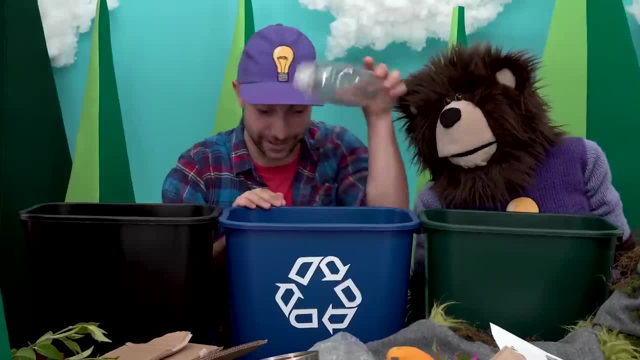 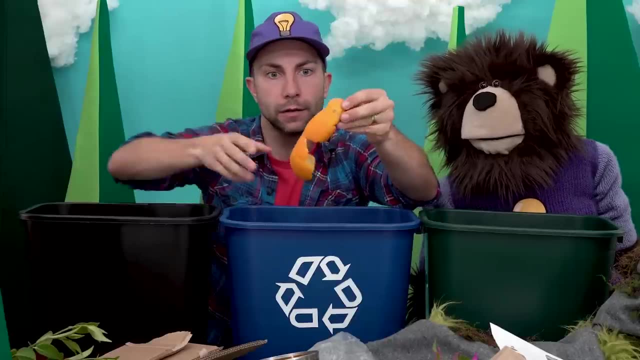 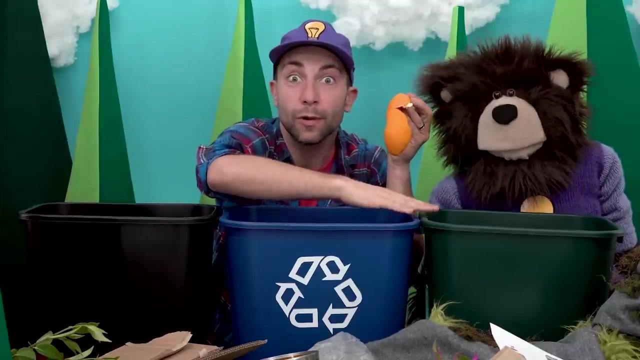 the blue bin. that's right, because you can recycle plastic. all right, so let's put that there. hmm, an orange peel. does this go in the green, blue or black bin? the green bin: that's right. you can put fruit scraps in the green bin. okay, what's next, mayta? 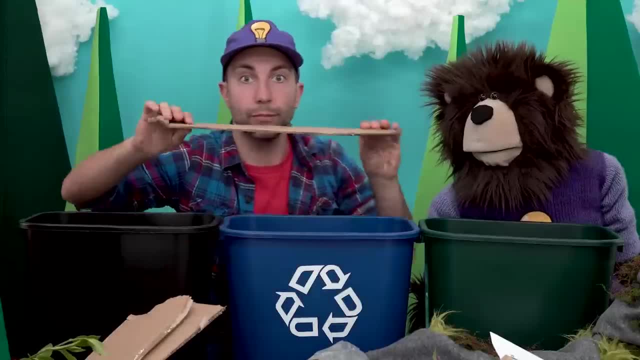 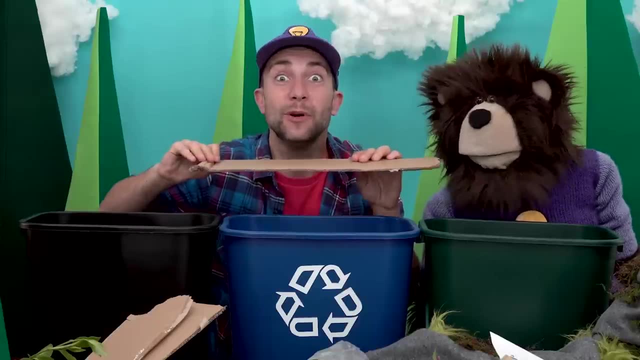 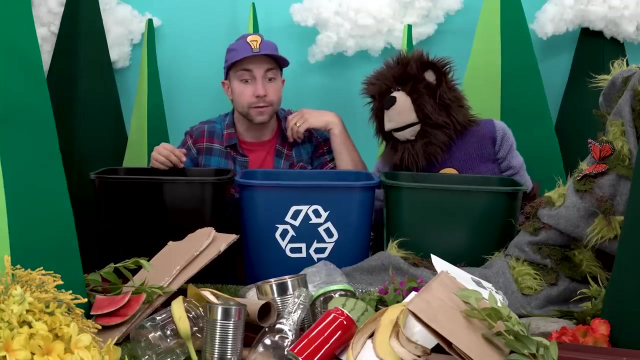 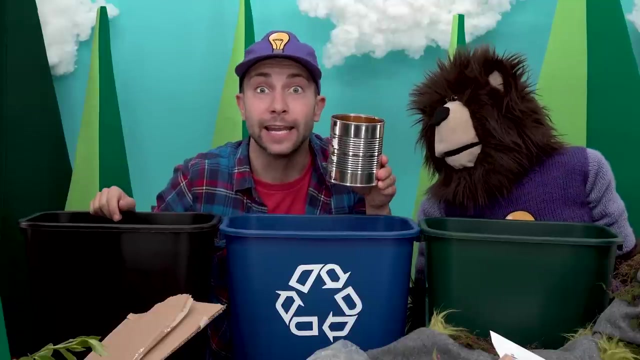 a piece of cardboard. does it go in the green bin, the blue bin, or the black bin? a blue bin, you're right, because you can recycle cardboard. all right, what else do we have? hmm, what is this? it's a tin can. can you recycle this tin can? 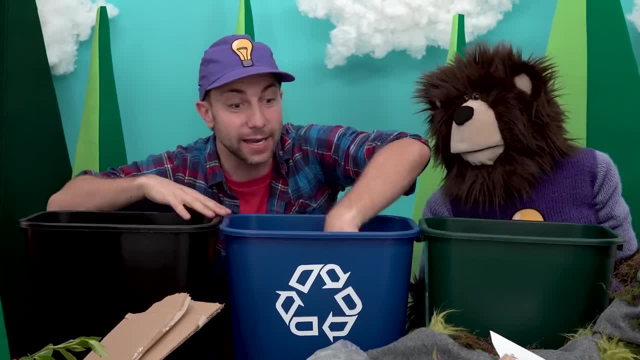 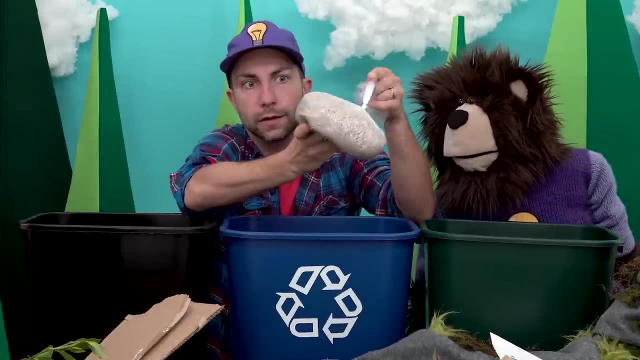 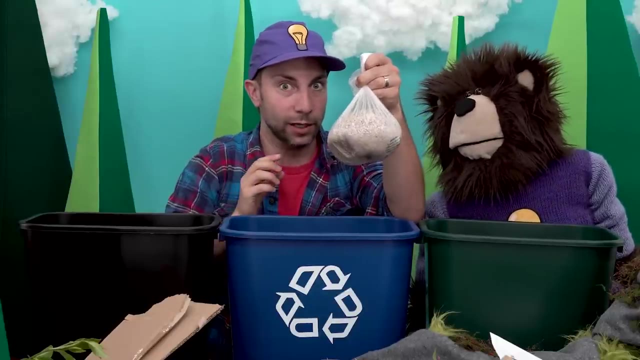 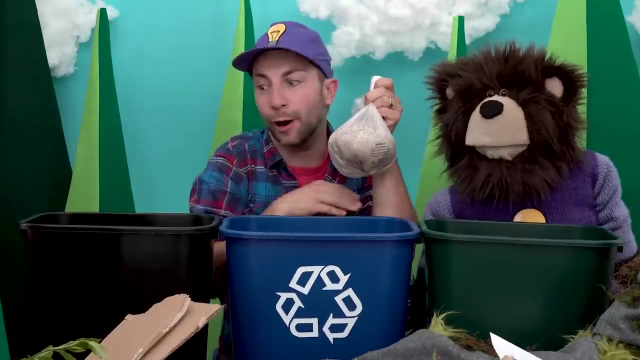 yes, you can. so we have to put it in the blue bin, all right. oh mayta, what is this? it looks like a bag of kitty litter. hmm, can we recycle this kitty litter? no. can we put it in the yard trimming bin? no, so it has to go in the- that's right, the black bin, all right. 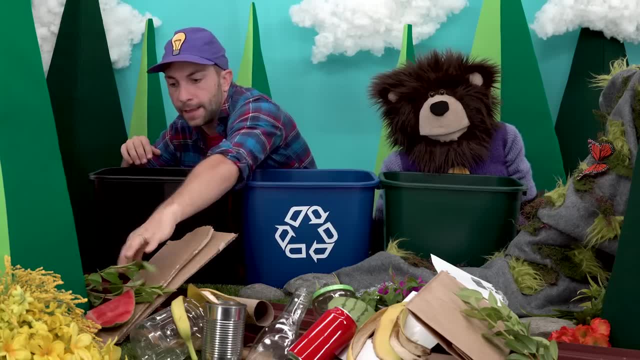 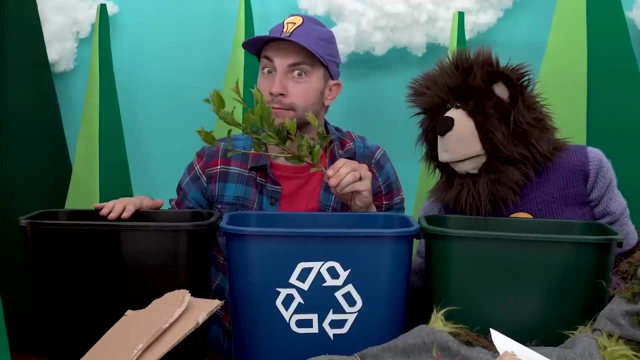 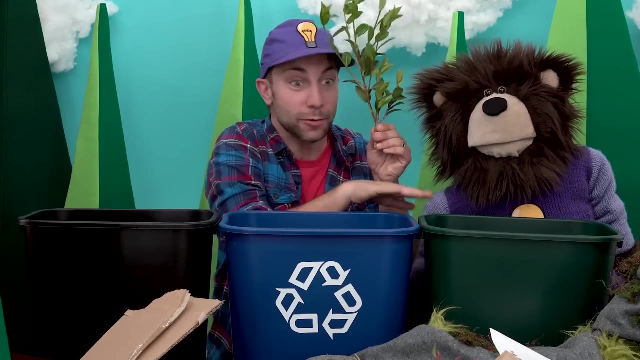 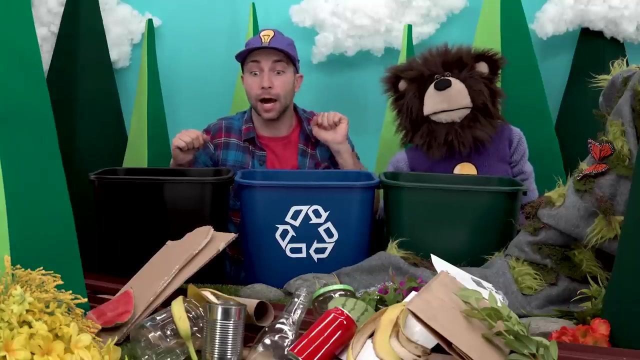 because it's trash, all right. so what else? hmm, i see this tree branch. where would this go? the black bin, no. the blue bin, no. so that leaves the green bin, that's right. goes right in the green bin, all right, where we are cleaning up. what else do we have? hmm, we have some mail, some paper. 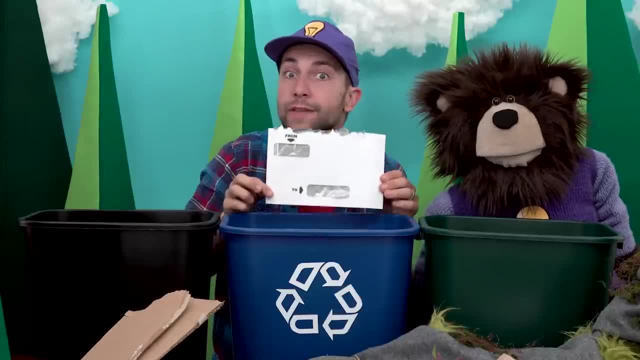 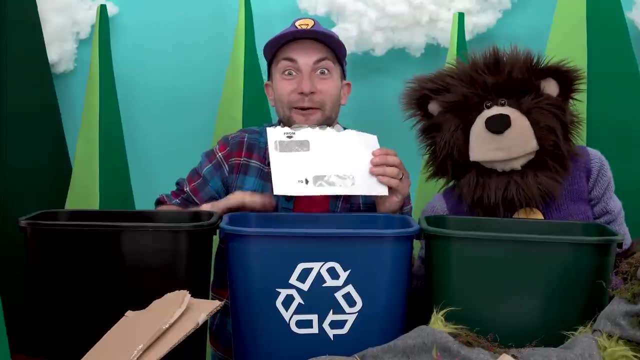 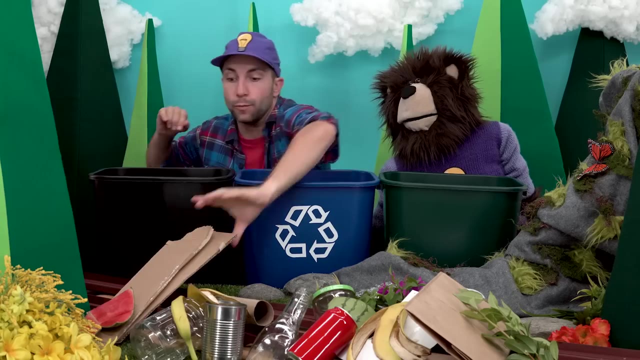 does this paper go in the trash or does it go in the recycling or does it go in the yard trimming bin? oh, mayta said it goes in the recycling bin, and he is right. you can recycle paper, so we'll put that right there. oh, we have some more cardboard. do you remember where the last piece of cardboard went? 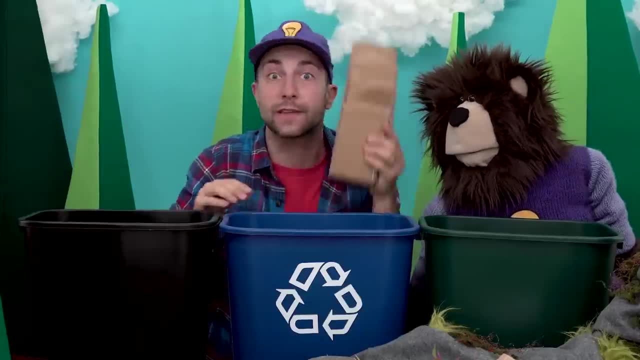 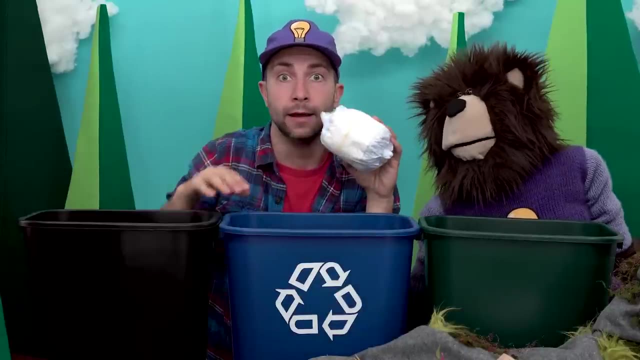 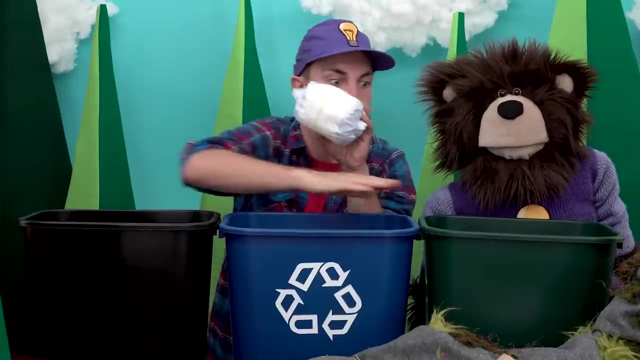 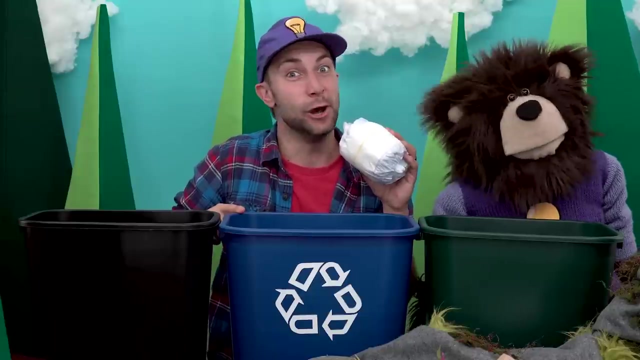 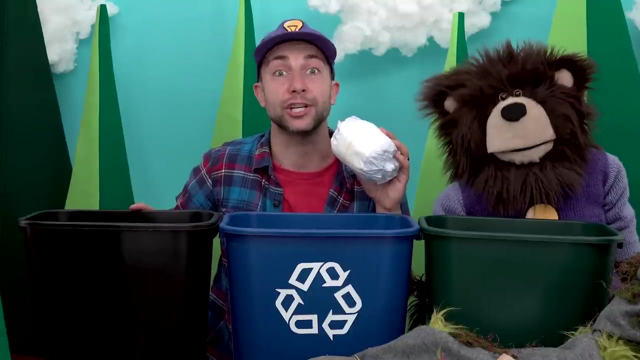 that's right. in the recycling bin you can recycle cardboard. okay. oh, mayta, we have a used diaper. where does this dirty diaper go? does it go in the yard trimming bin? no, does it go in the recycling bin? no, so it must go in the black bin. yes, the trash. okay, we are cleaning up. oh. 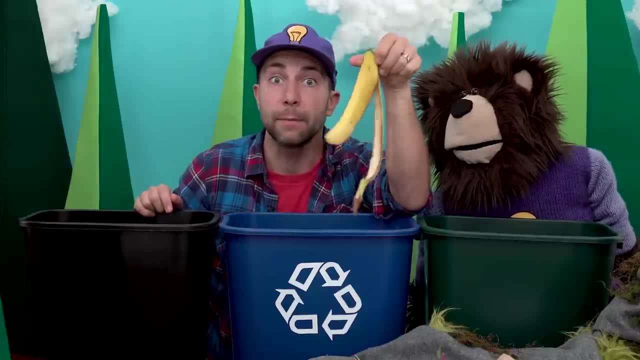 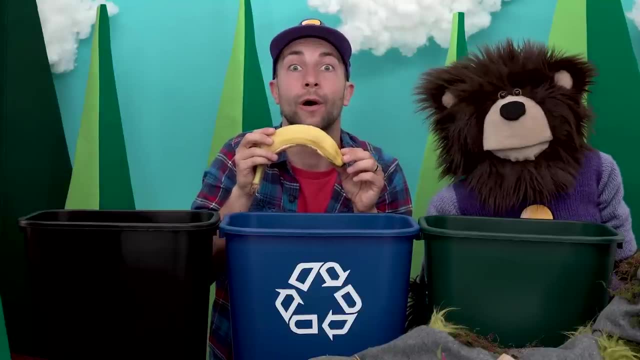 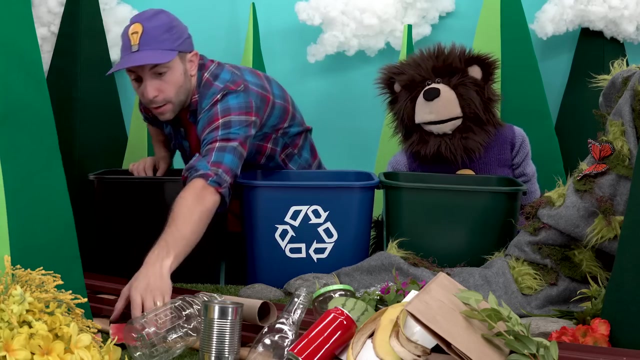 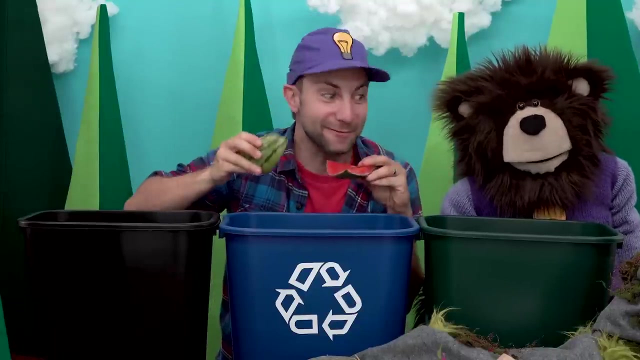 look at this, mayta, a banana peel. now that looks like fruit scraps. where do fruit scraps go? you're correct, the green bin, okay, let's see. oh look, we have two more fruit scraps. so where do these go? that is right, and you are right too, mayta, the green bin, okay. 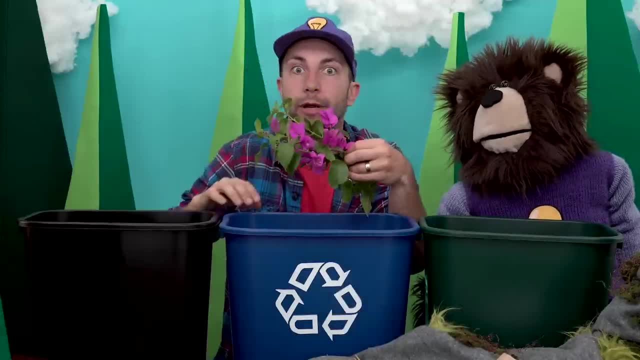 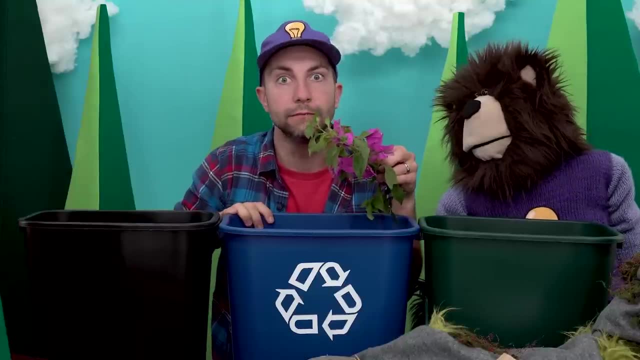 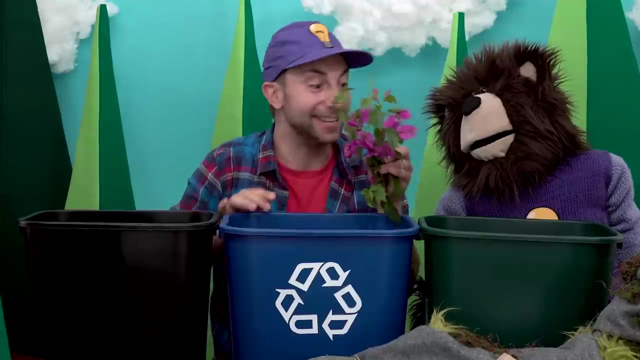 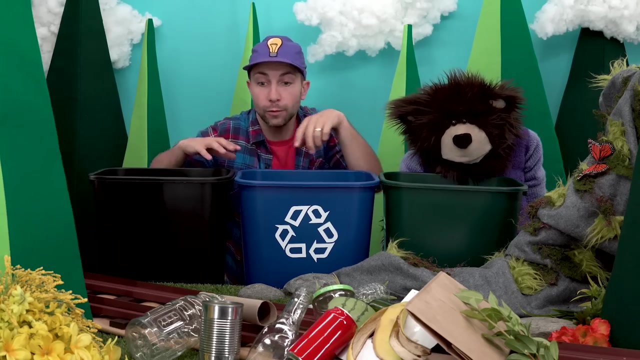 we have some flowers right here. they're very pretty. where do they go? the black bin, no, because they're not trash. the blue bin: no, we can't recycle the flowers. that's right, they go in the green bin. okay, let's drop them in. okay, what do we have here? oh look, it's another plastic bottle. it's another plastic bottle. 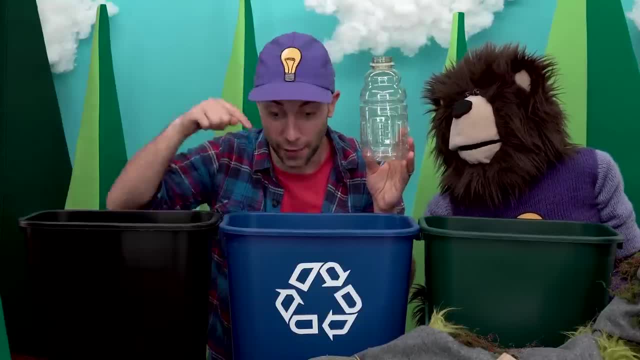 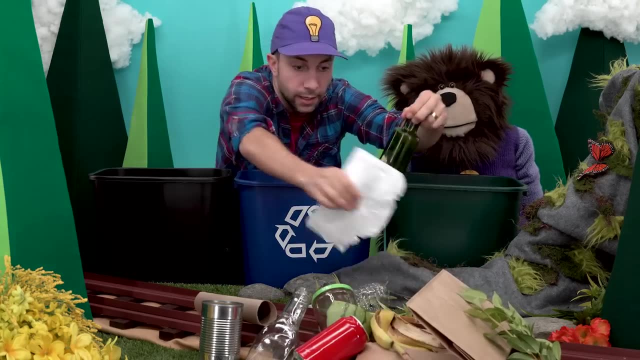 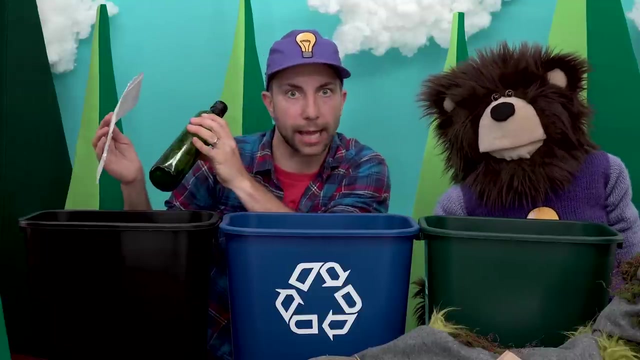 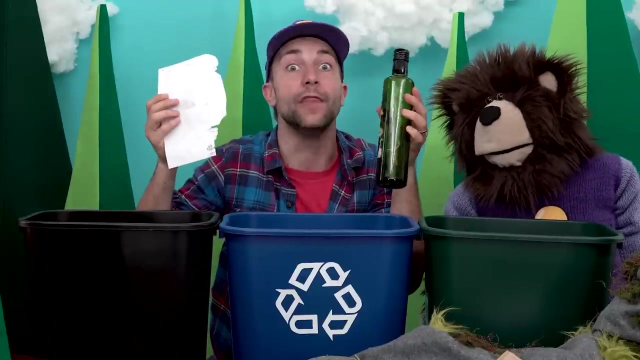 you are right, the blue bin. you can recycle plastic. okay, let's keep going. oh look, mayta, we have a piece of paper and a glass bottle. now are these trash? do they go in the black bin? no, are they yard trimmings? no. so that leaves the blue bin. yes, glass and paper can be recycled. 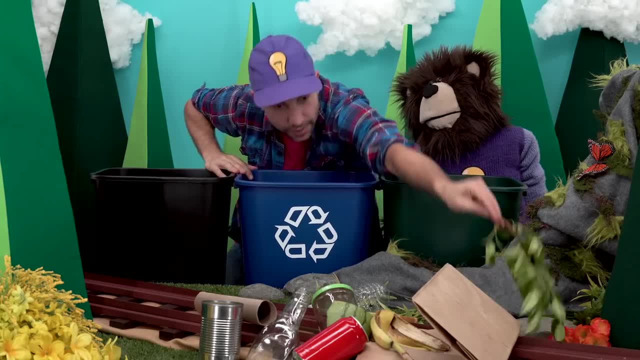 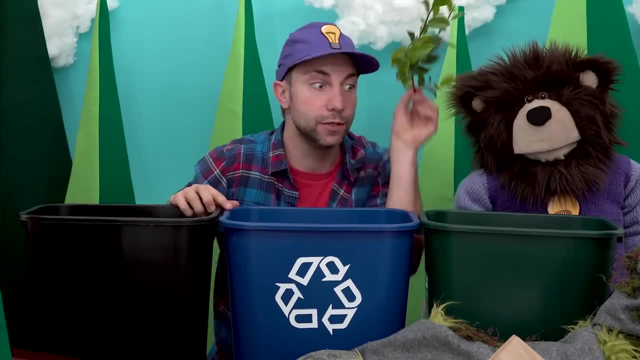 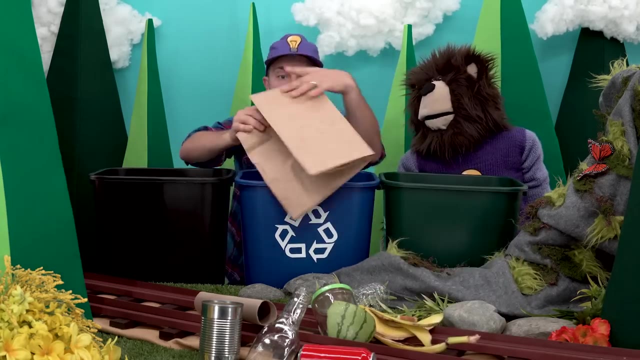 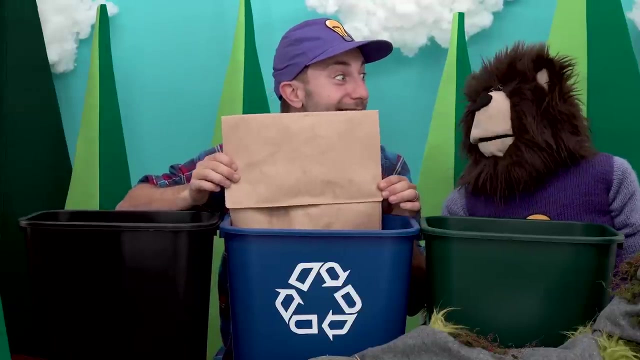 okay. so we're moving on to this tree branch. where does the tree branch go? that's right. the green bin into yard trimmings? okay, let's keep cleaning up, mayta. okay. so we have a brown paper bag. where does paper go? do you know, mayta? yeah, where does it go? 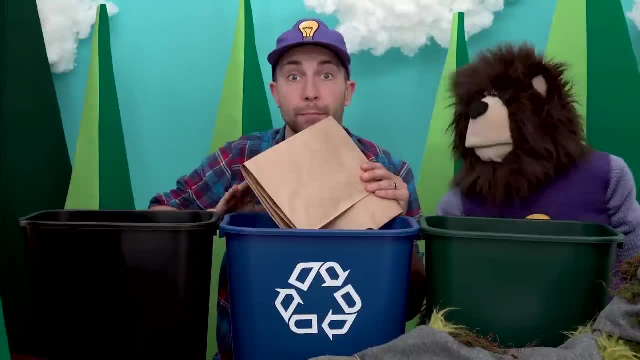 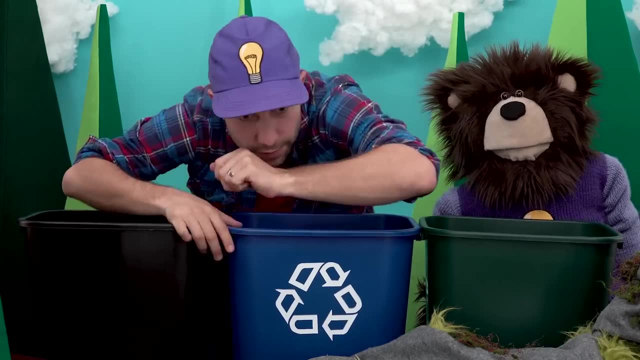 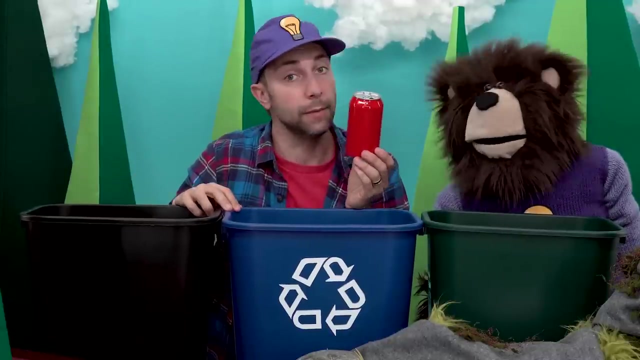 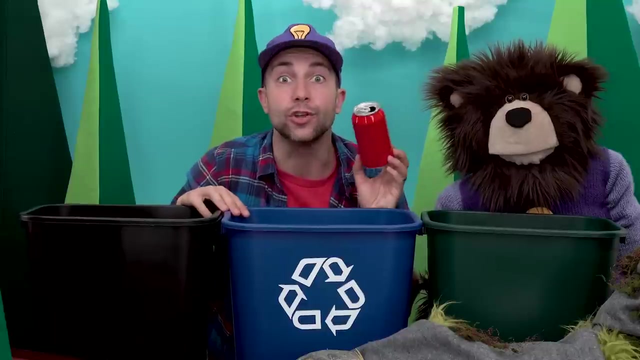 you are correct, it goes in the blue recycling bin because you can recycle paper. all right, so let's put that right in there. and oh, let's stretch way out here. oh, it's another soda can, or maybe you call it a pop can. where does this go? that's right, the blue bin, because you can recycle aluminum cans. 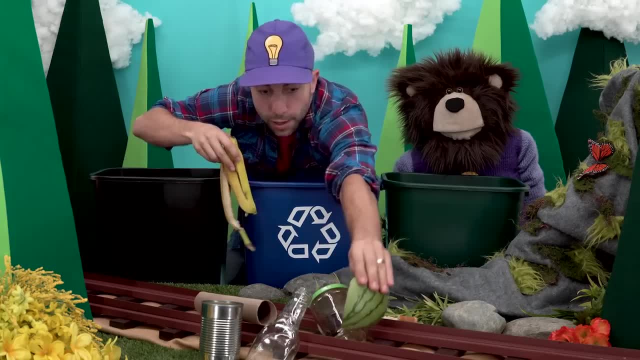 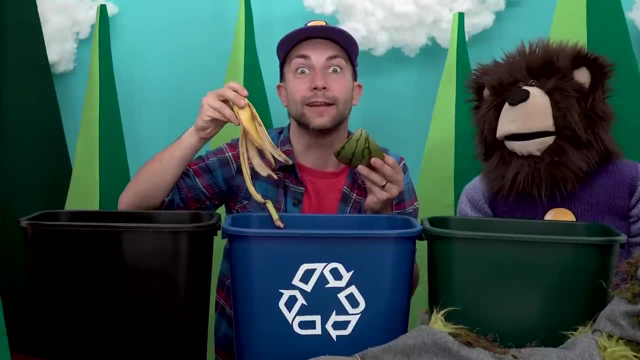 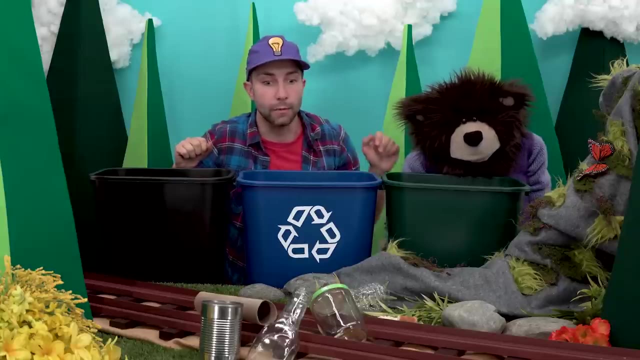 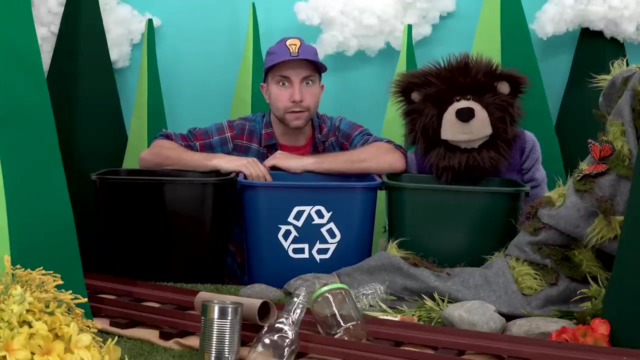 all right, all right, so we have some more fruit scraps. where do they go, mayta, that is correct. fruit and veggie scraps can go in the green bin, all right. oh, mayta, it looks like there is a half-eaten sandwich, do you see it? it's right over here. 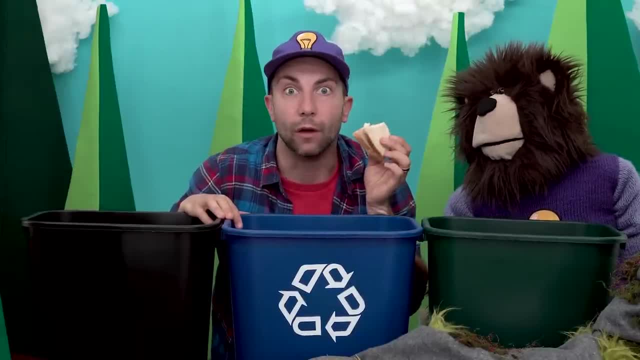 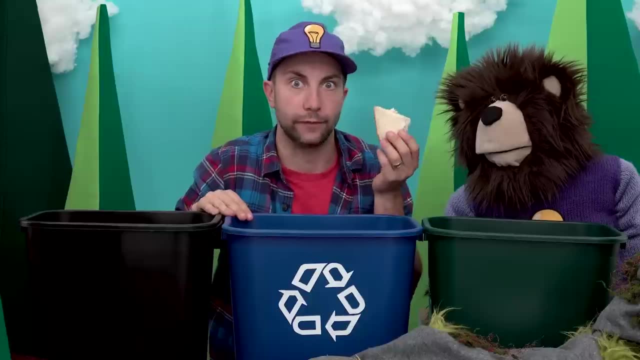 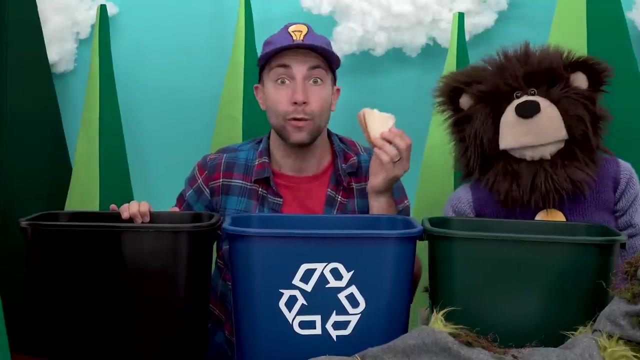 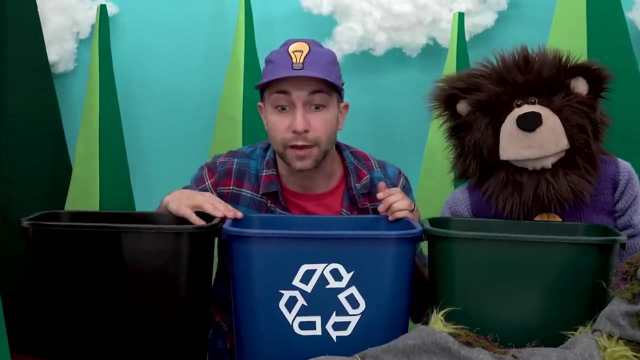 hmm, where does this go? does it go in the green bin? no, can you recycle a half-eaten sandwich? no, so that leaves the black bin. so we will put our little piece of leftover sandwich in the trash. okay, what do we have left? okay, we have another tin can. where does the tin can go? 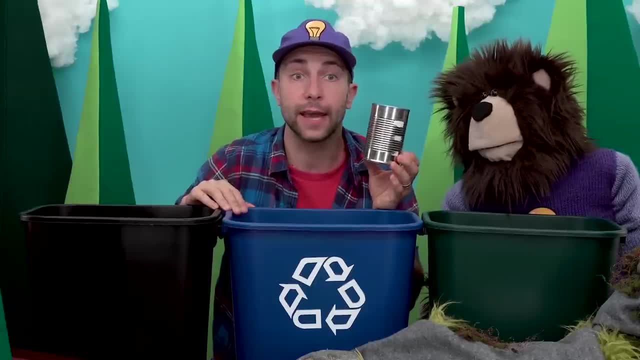 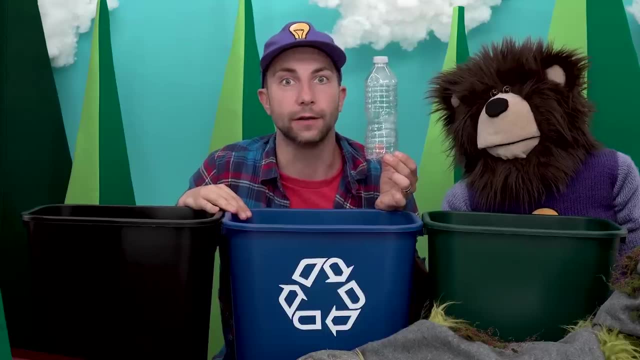 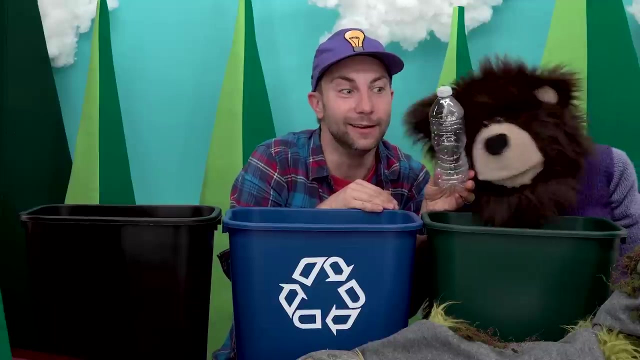 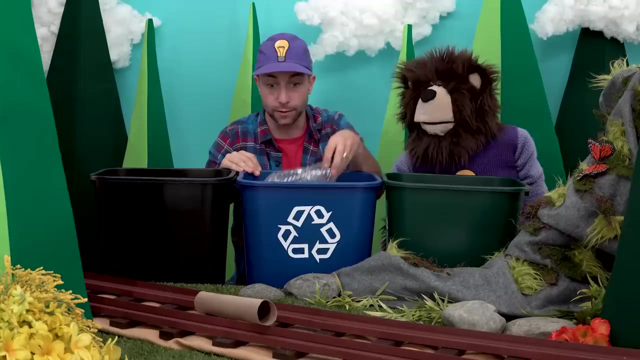 that's right. the blue bin, because tin cans can be recycled. woo, woo, woo. all right, okay, and a plastic bottle. where does this go? the black bin? no, the green bin. oh, mayta is saying it goes in the blue bin. well, you are right, you can recycle plastic. so we put. 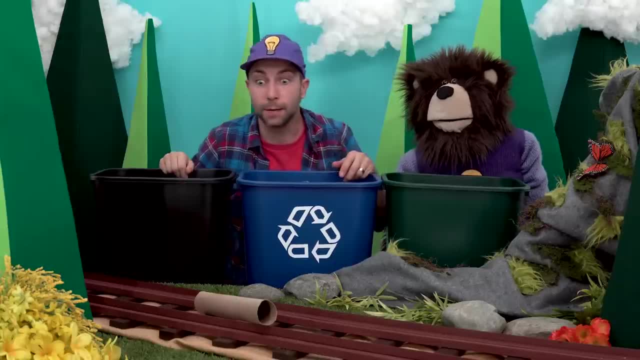 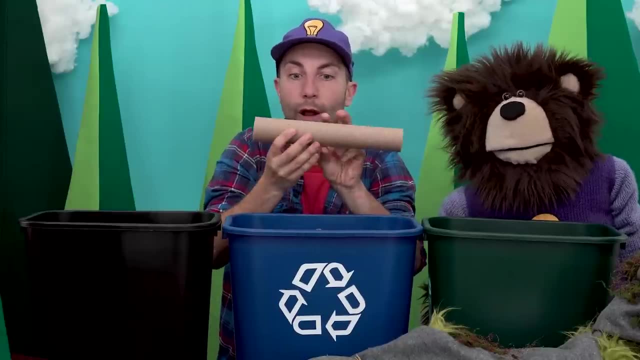 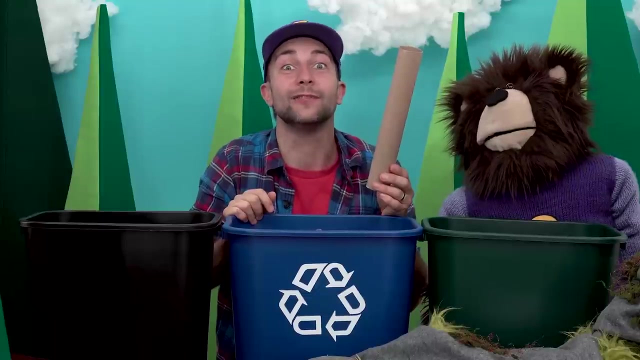 that in there, mayta, we are almost done cleaning up. we have one thing left. it's a paper towel roll. it's made out of a plastic bottle. it's a paper towel roll. its made out of of cardboard. where does this go? that is right, the recycling bin. we can recycle. 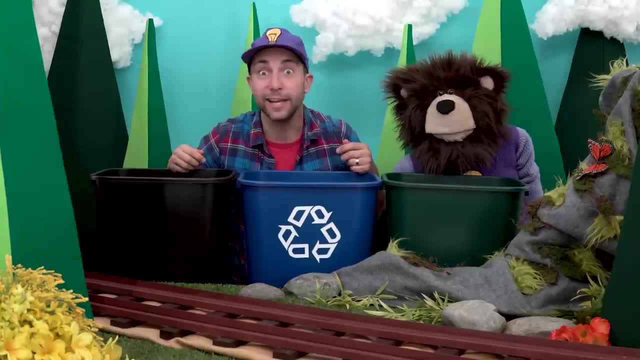 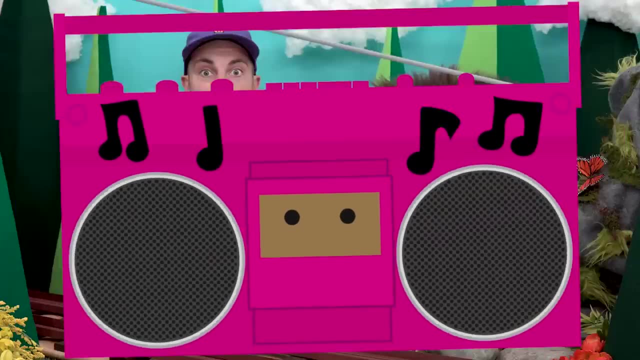 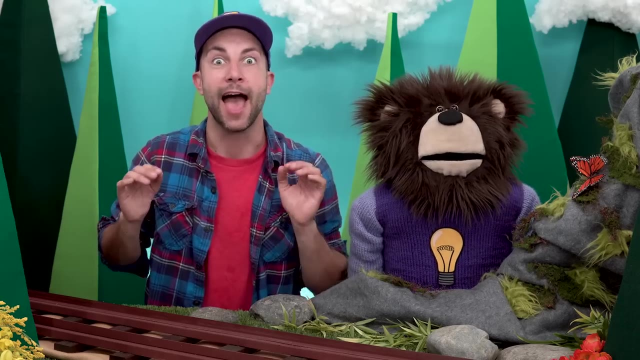 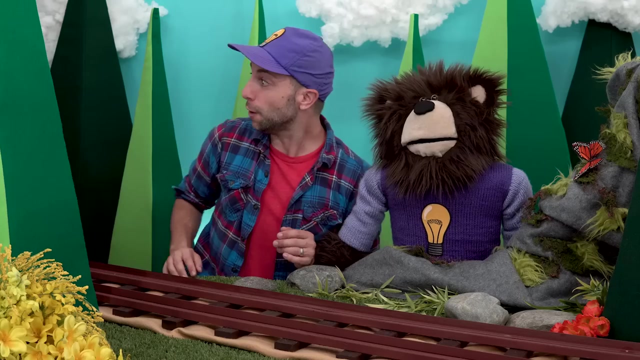 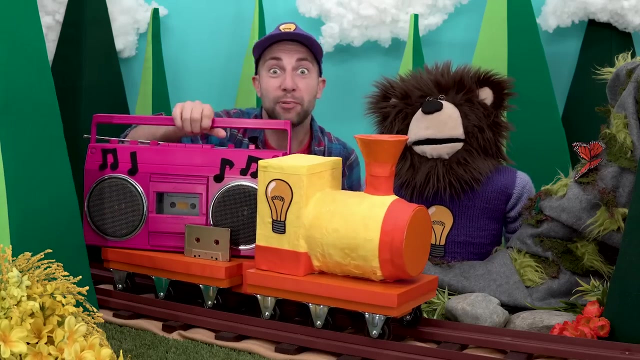 this. wow, we cleaned up everything on the train tracks. thank you so much for your help. you know what time it is. it's time to dance. this is where we stop what we're doing. stand up and dance. you can do whatever dance move you feel like doing. oh, look, it's the idea train. oh, it's pinky the boom box. hi, pinky the.